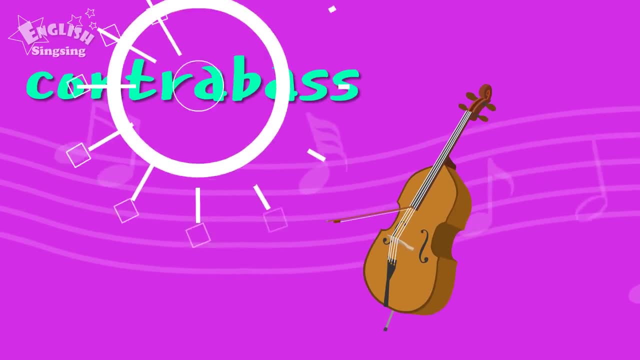 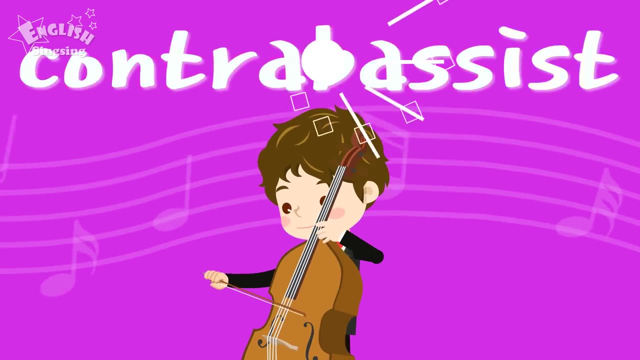 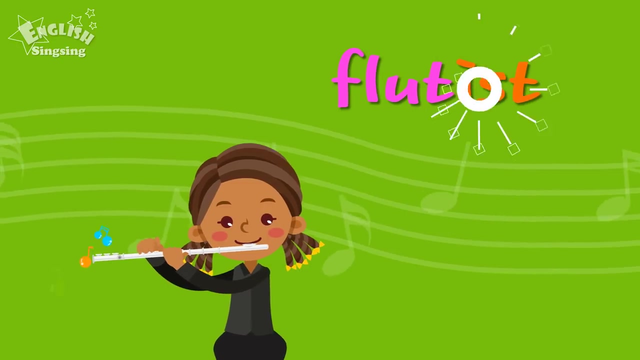 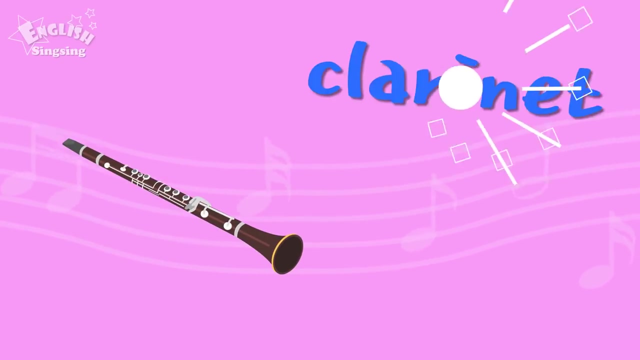 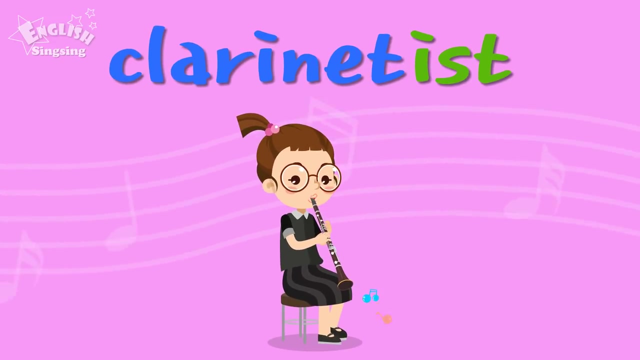 cellist. contrabass, contrabassist, contrabassist- He is a contrabassist, contrabassist. flute, flute, flutist. She is a flutist. flutist, clarinet, clarinet, clarinetist. She is a clarinetist, clarinetist. 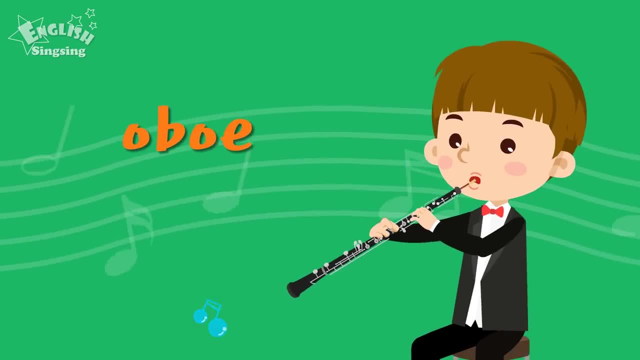 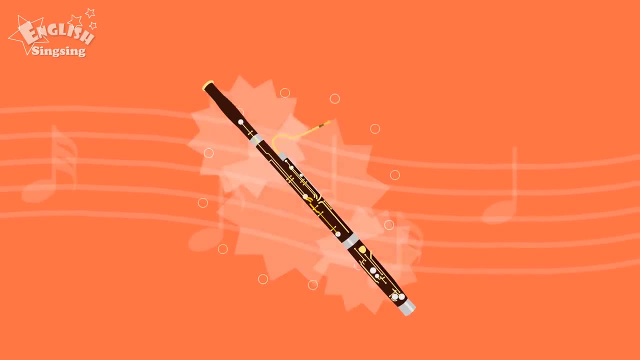 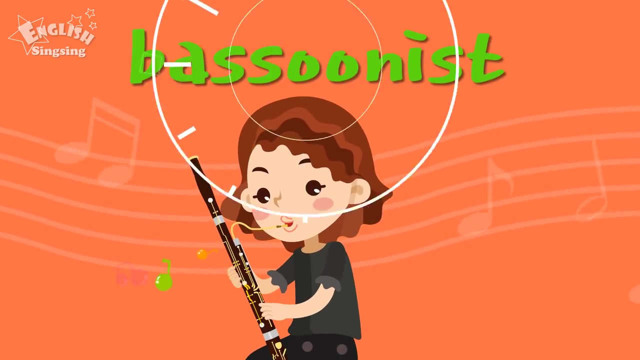 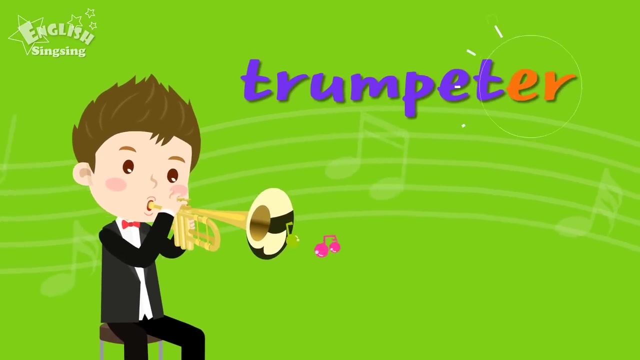 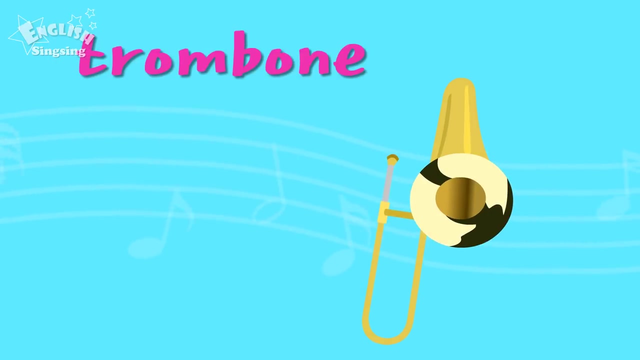 oboe, oboe, oboist. He is an oboist. oboist. bassoon, bassoon- bassoonist. She is a bassoonist. bassoonist. trumpet trumpet, trumpeter trumpeter. He is a trumpeter trumpeter- trombone. 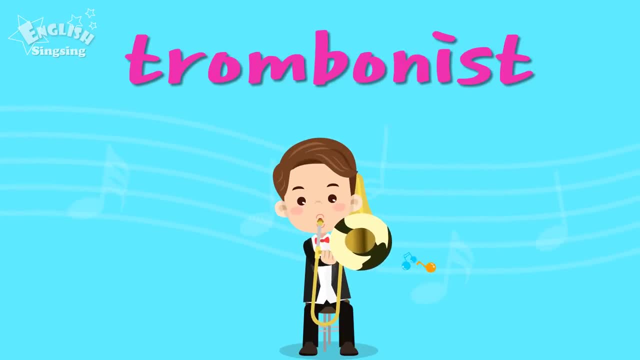 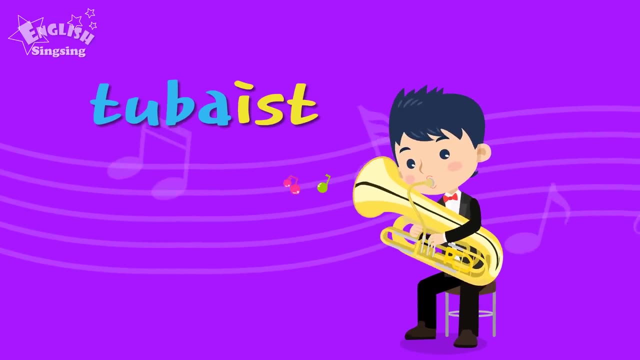 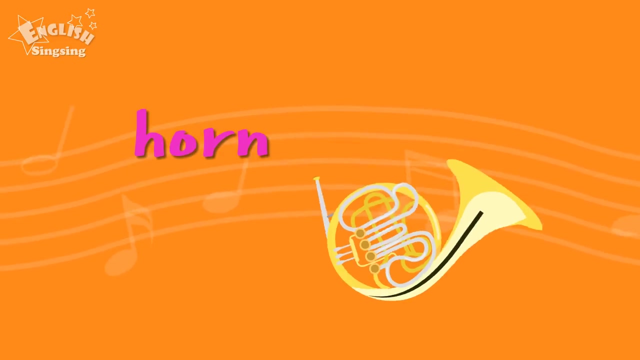 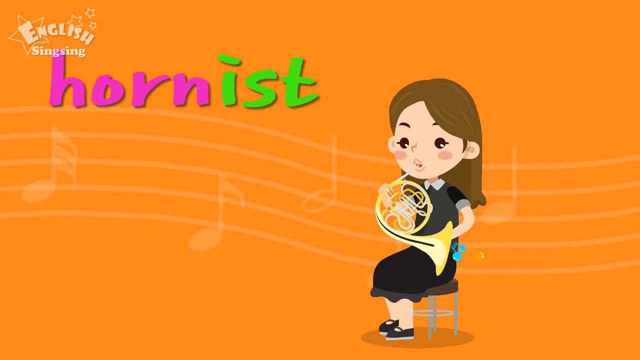 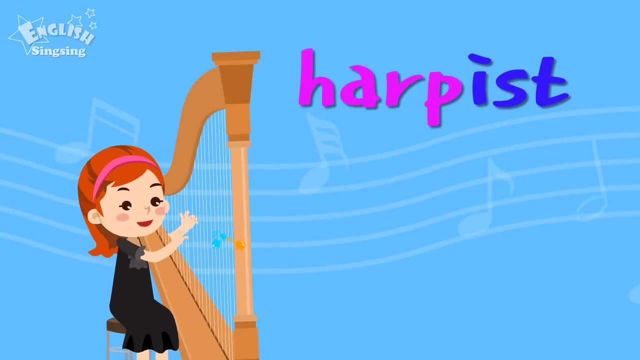 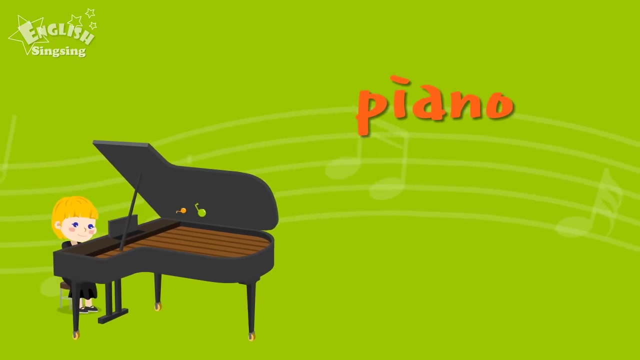 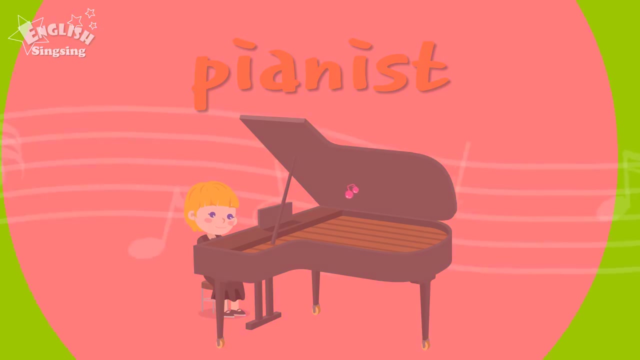 trombone, trombonist, trombonist, tuba, tubaist, tubaist. He is a tubaist tubaist. horn hornist hornist. She is a hornist hornist. harp harp, harpist, harpist, harpist. 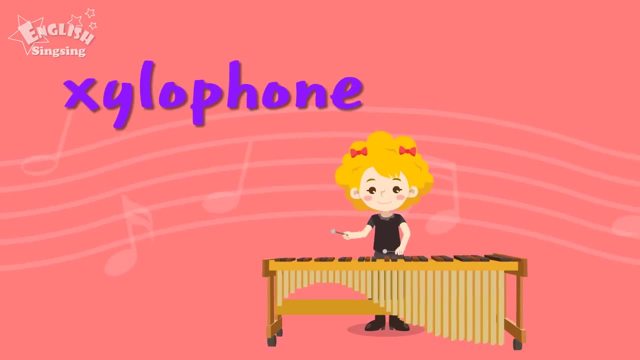 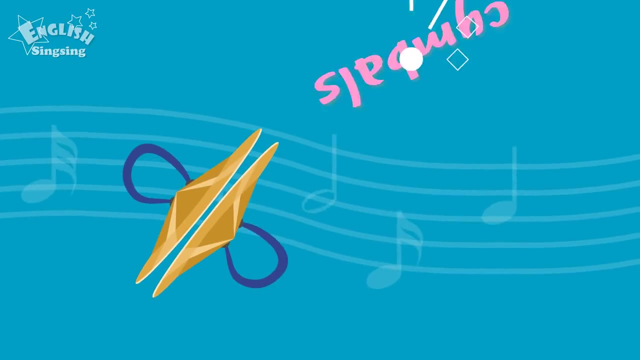 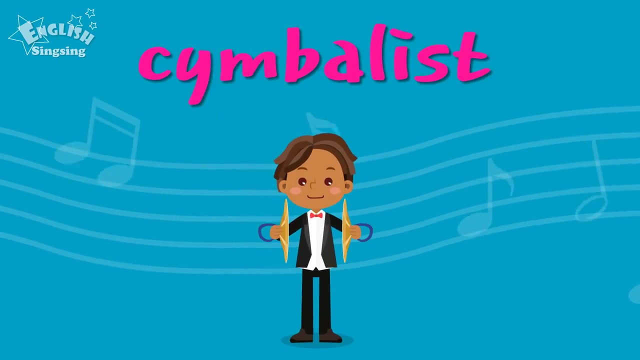 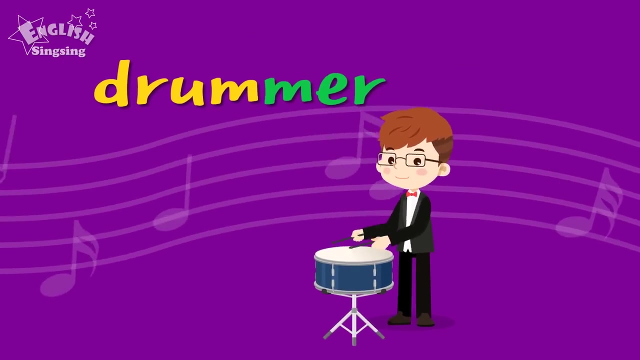 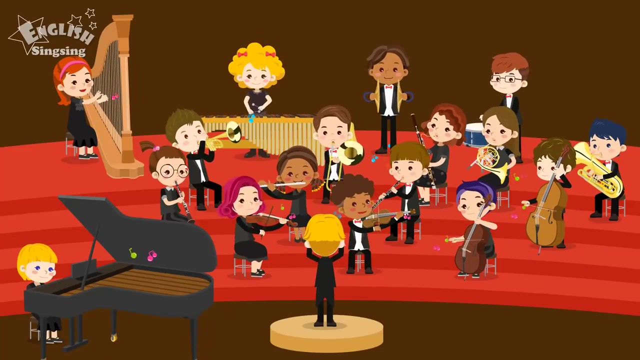 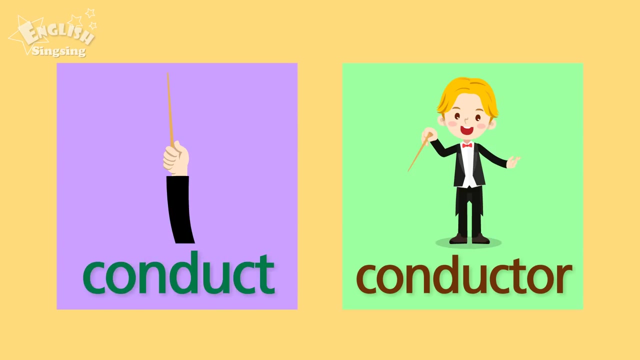 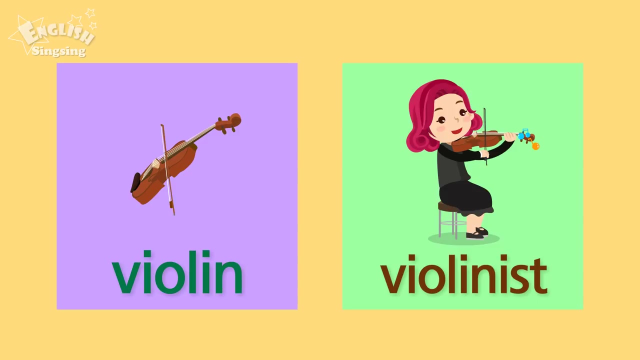 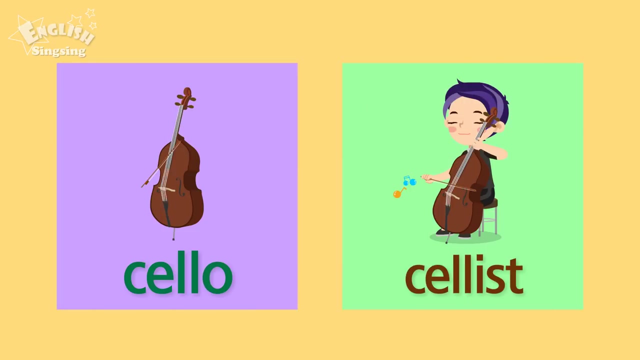 harpist. harpist xylophonist: She is a xylophonist. symbols, symbolist: He is a symbolist. drum drummer: He is a drummer review conduct. conductor: violin, violinist, viola, violist cello, cellist contrabass.